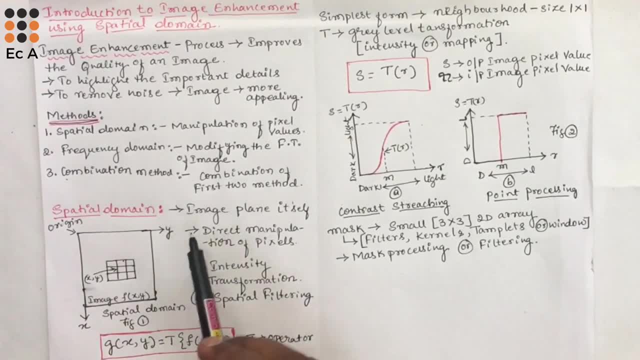 The image processing in this domain is direct manipulation of pixel values. So the image processing in this domain is direct manipulation of pixel values, pixel values of an image. There are two categories of spatial domain. First one is intensity transformation, in which the modification of intensity values of pixel will take place. 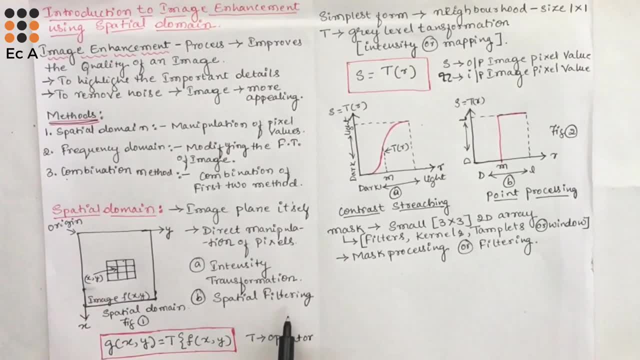 and second one is spatial filtering. Here there will be direct manipulation of pixels using a mask. The spatial domain technique operates directly on the pixels of an image, but in frequency domain operations are performed on Fourier transform of an image. So this is the difference between spatial domain and frequency domain. The spatial domain process is denoted by: 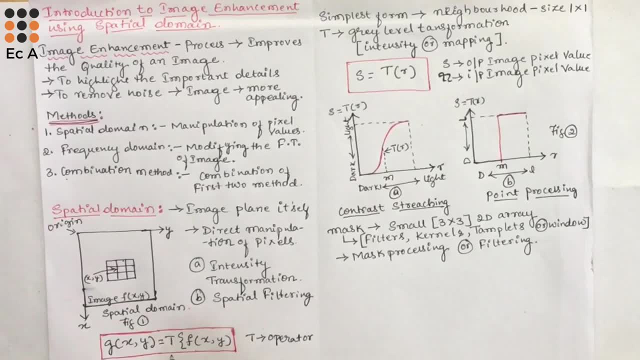 g of x comma y will be equal to t of f of x comma y. Here f of x comma y will be equal to t of f of x comma y. Here f of x comma y will be equal to t of f of x comma y. 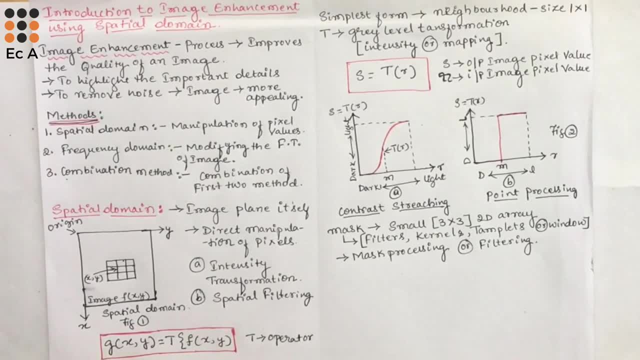 Here, f of x comma y is an input image and g of x comma y is the output image, and the term t is known as the operator. This operator can be applied to the single image or to the set of images. This figure shows the basic implementation of this equation on a single image, which means: 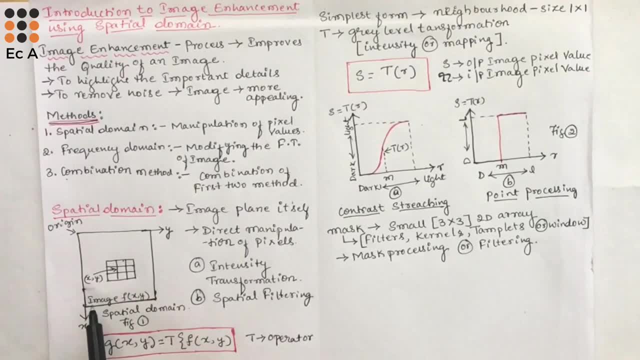 the operator is applied on a single image. The point x comma y is the arbitrary location in an image and the region next to this pixel is known as neighborhood of this pixel x comma y In spatial domain processing. the spatial domain process consists of moving the origin of the neighborhood from pixel to pixel and applying the operator t. 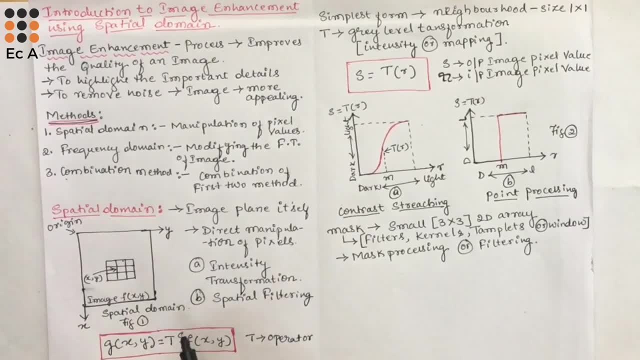 to the pixel in the neighborhood that will be yielding the output of the location. If we consider this pixel with the neighborhood pixel, so this will be moved from this origin and the operation is performed on this. based on the operator, And once the operation is performed, 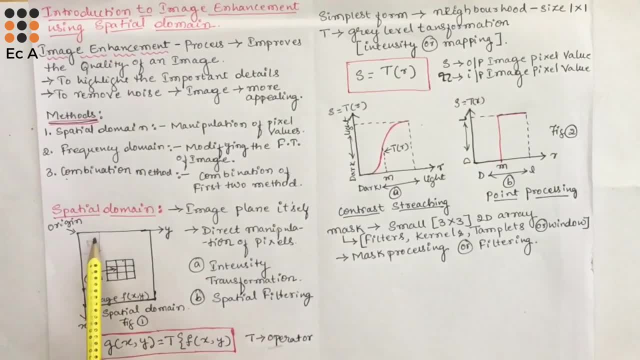 this pixel x comma y, along with the neighborhood, will be moved to the next pixel value and then the operation will be performed again. Likewise, this operation will be performed on entire pixel of the image. The simplest form of t will be performed on operator x comma y. Now the next step is to express the scale of an image. So in this, 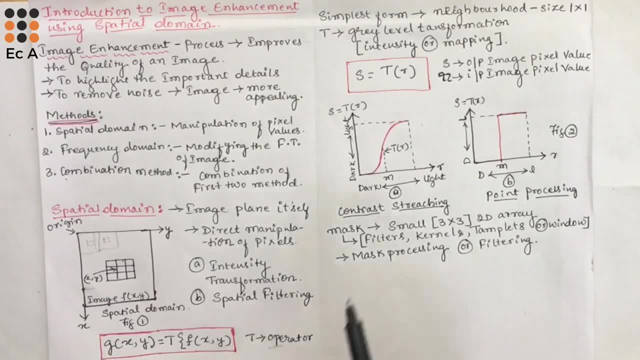 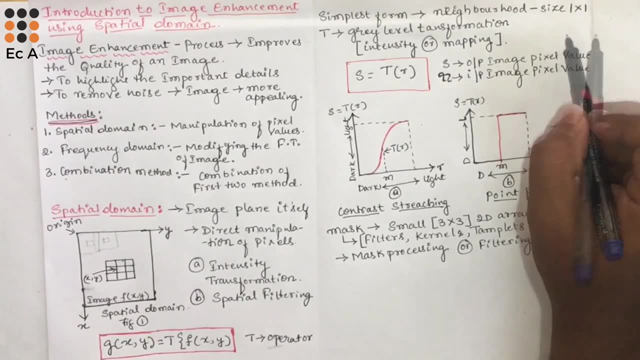 case, instead of when the number of pixels is zero, so that why the number of pixels is zero? when the number of pixels is equal to zero, we will work on all the values: M equals z minus i power. omega x minus i square plus i du square plus i square plus i square. 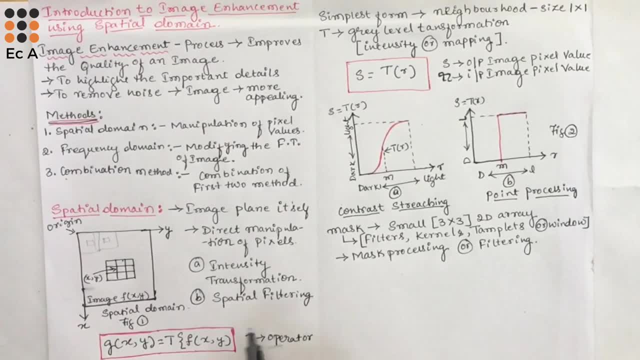 times the number of pixels and make the project complete. The next step is to incorporate a linear and half circel thing to the Jaechen general error. we can use the product rules, So if d is a컵 and d left one such function. 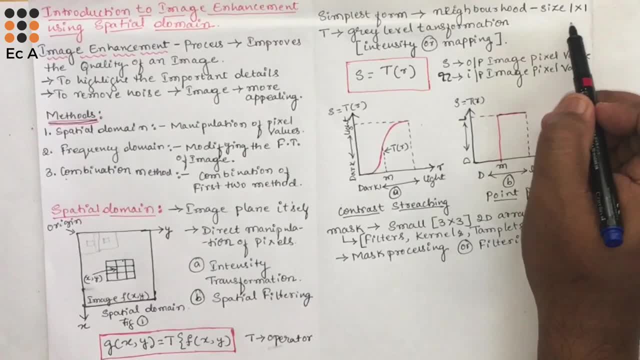 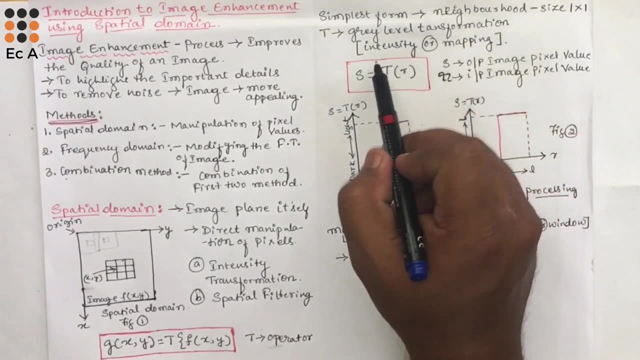 styling. If d becomes a, well that the element is a H, seen, discover, developed by a Frederik D, the gray level, if we take the neighborhood of size 1, cross 1.. Hence we will call T as gray level, transformation, or it is also known as intensity transformation or mapping. 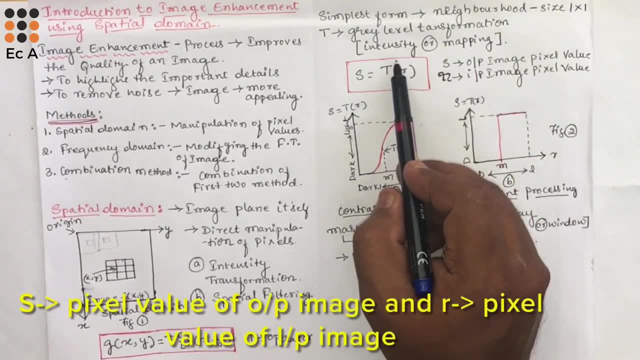 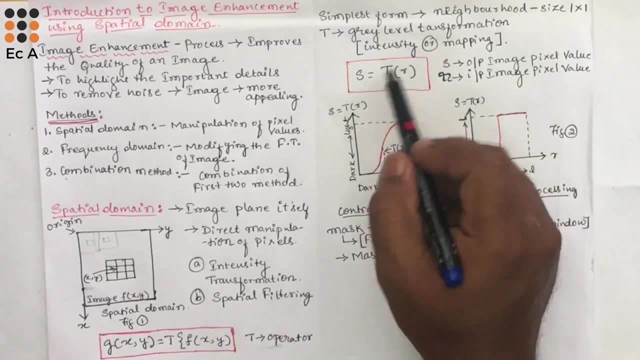 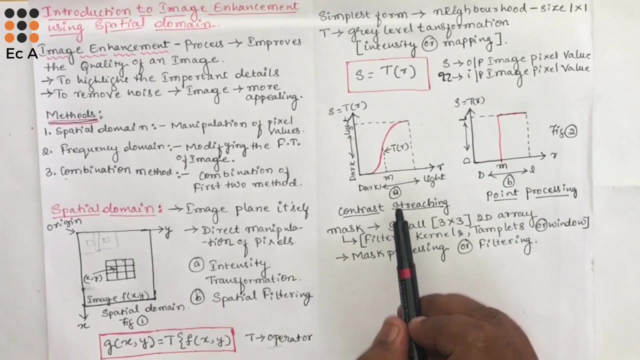 This gray level transformation, or intensity level transformation, can be denoted as: S is equal to T of r and T is the operator. These two figure shows the gray level transformation. Figure A shows the effect of transformation that would produce an image of higher contrast than the original image. This is the transformation that shows the image that is of higher contrast. 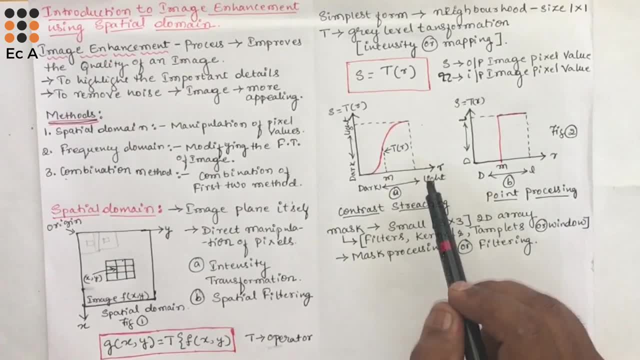 compared to the original image. In this transformation, the region of the image will be darken below M and it will be brightening the level above M. This technique is also known as contrast stretching. The value of r below M are compressed by transformation function. 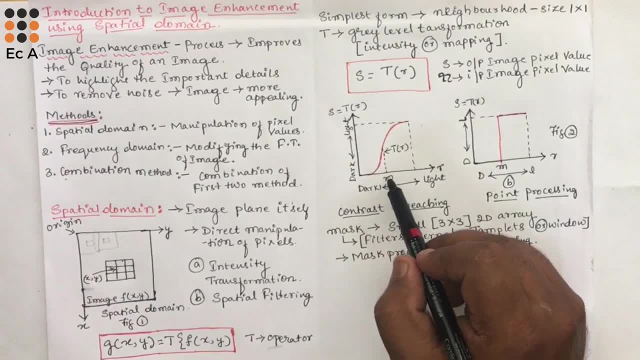 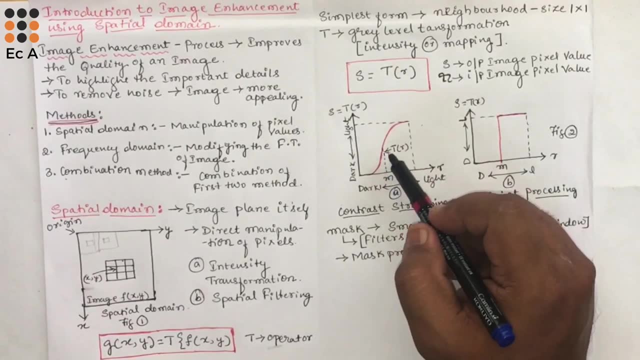 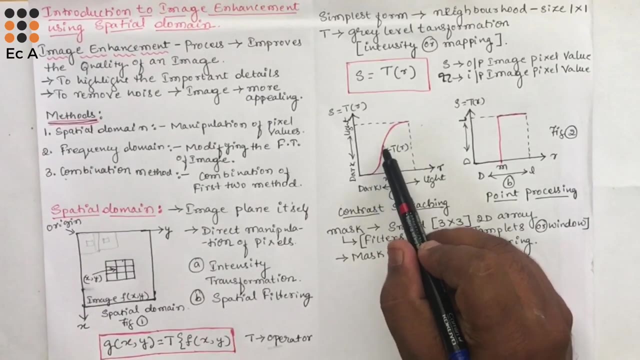 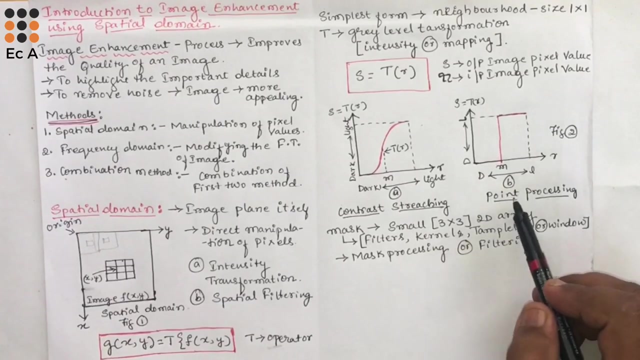 into a narrow range of S and the value of r above M are compressed by the transformation function towards lighter region. If you observe in this graph, the transformation from dark to light is having a form of a curve that represents the contrast stretching. Figure B shows the transformation T of r that produces two level image.